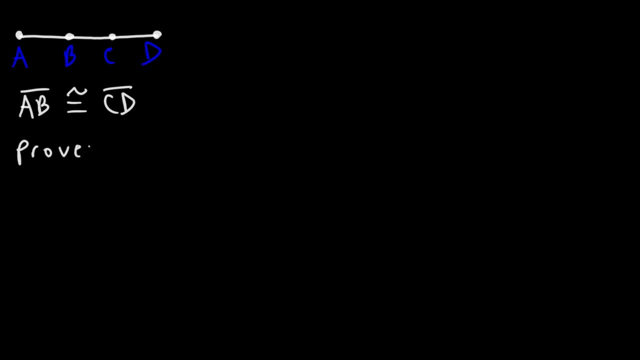 Our task is to prove that segment AC is congruent to segment BD. Go ahead and try that. So let's create two columns. We're going to put the statements in the first column and then the reasons for those statements in the second column. 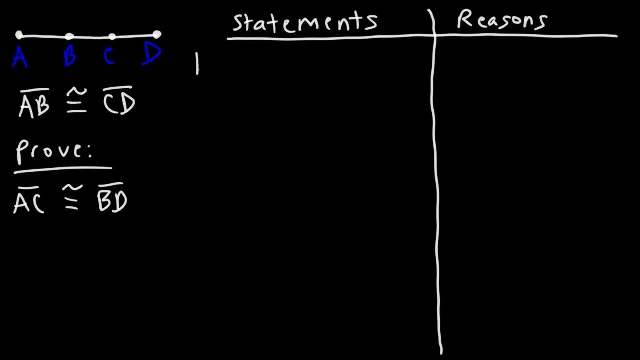 Now the first thing we should write as our statement is what's given, That is, segment AB is congruent to segment CD, And that's a given. Now what's the next step that we can do? The next step is sort of a formality. 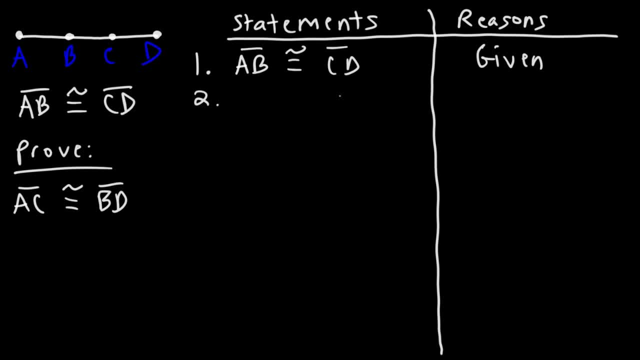 If segment AB is congruent to segment CD, then mathematically speaking we could say that AB is equal to CD. Now what's the reason for this? What can we put in the second column For this situation? you can say: definition of congruent segments. 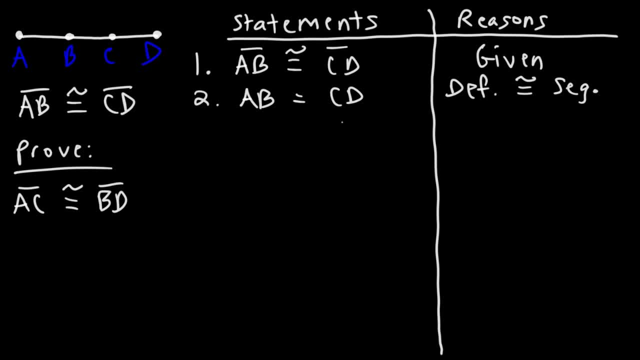 So I'm not going to write the whole sentence out, just to conserve space. but you get the point. Now let's move on to number three. So let's talk about what we're trying to do. We're trying to prove that AC, which is this part. 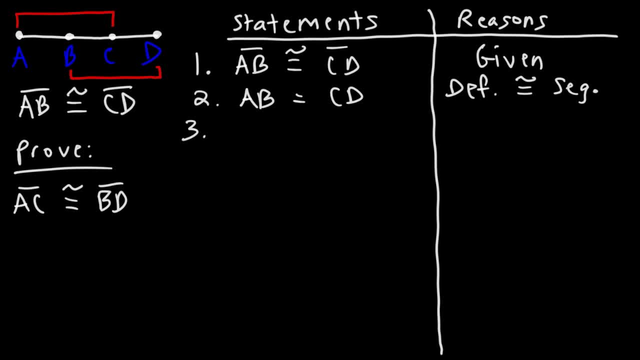 is congruent to BD. We know that AB is equal to CD, So the only part that's missing is BC. Notice that AB plus BC will give us segment AC And BC plus BD will give us- I mean, BC plus CD will give us BD. 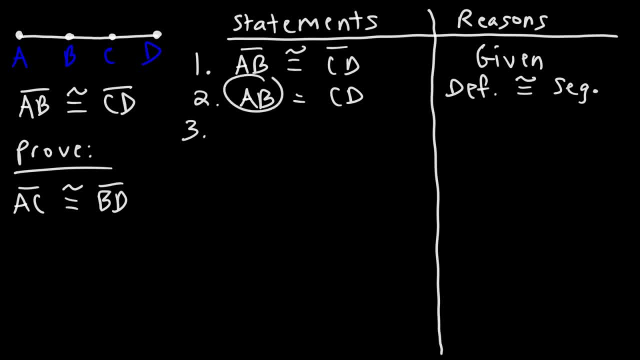 So this tells us that we need to add BC to both sides of this equation. But before we do that, let's write down another formality. We're going to say that BC is equal to BC based on the reflexive property. 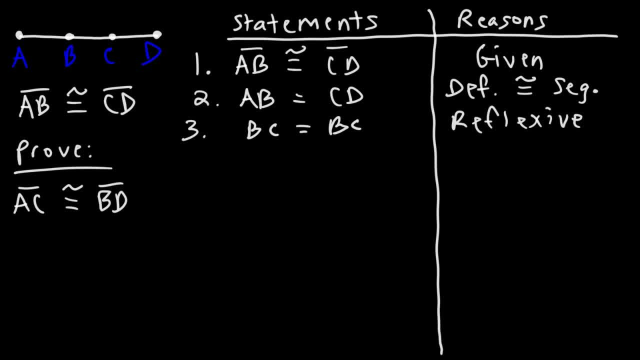 Now you might be wondering: why do we need to do that? Some teachers may require it, others may not, but just in case, we're going to put that there. So now we're going to add statements two and three And we're going to write down the equations for it. 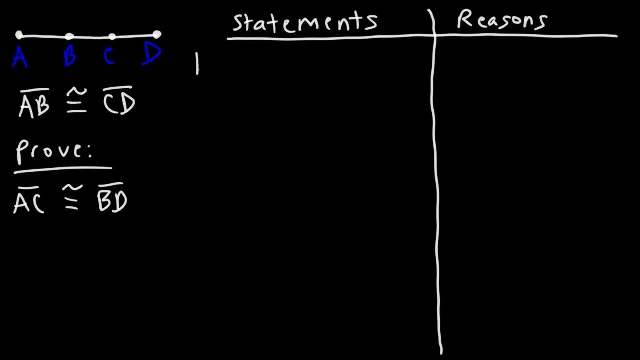 Now the first thing we should write as our statement is what's given, That is, segment AB is congruent to segment CD, And that's a given. Now what's the next step that we can do? The next step is sort of a formality. 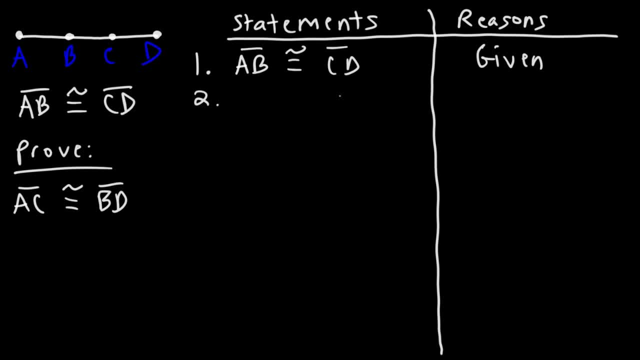 If segment AB is congruent to segment CD, then mathematically speaking we could say that AB is equal to CD. Now what's the reason for this? What can we put in the second column For this situation? you can say: definition of congruent segments. 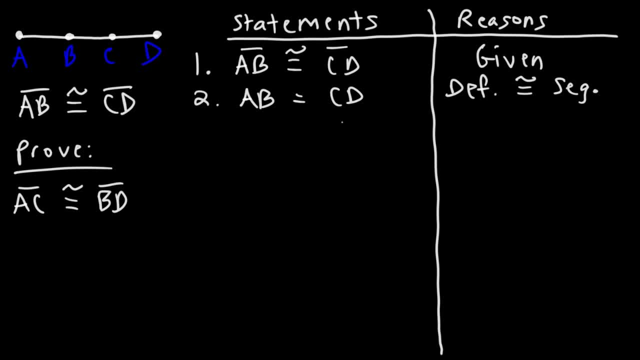 So I'm not going to write the whole sentence out, just to conserve space. but you get the point. Now let's move on to number three. So let's talk about what we're trying to do. We're trying to prove that AC, which is this part. 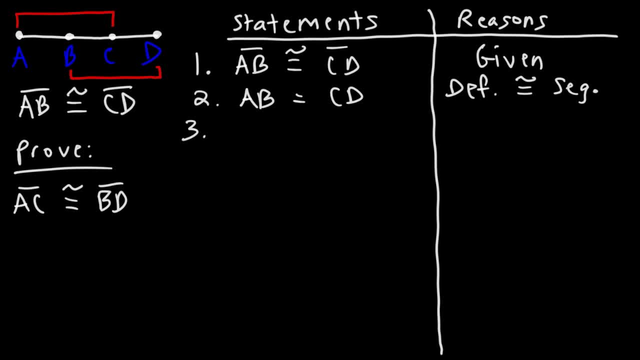 is congruent to BD. We know that AB is equal to CD, So the only part that's missing is BC. Notice that AB plus BC will give us segment AC And BC plus BD will give us- I mean, BC plus CD will give us BD. 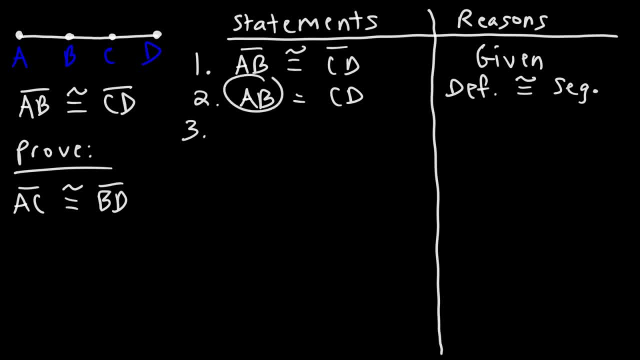 So this tells us that we need to add BC to both sides of this equation. But before we do that, let's write down another formality. We're going to say that BC is equal to BC based on the reflexive property. 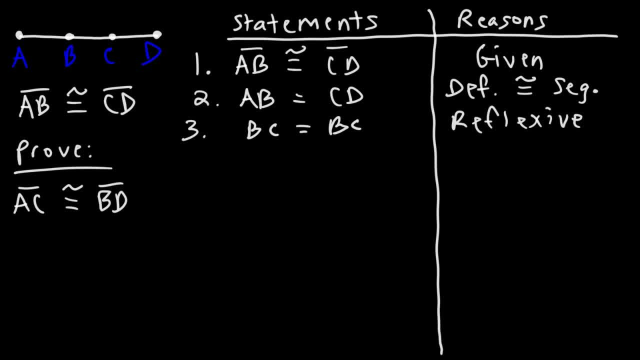 Now you might be wondering: why do we need to do that? Some teachers may require it, others may not, but just in case, we're going to put that there. So now we're going to add statements two and three And we're going to write down the equations for it. 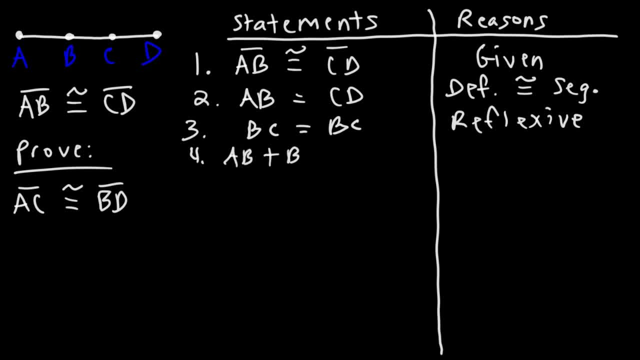 So we're going to get AB plus BC. basically add in the left side and add in the right side. of the two equations We're going to get that's going to equal BC plus CD. Now this is basically the addition. property of equality. 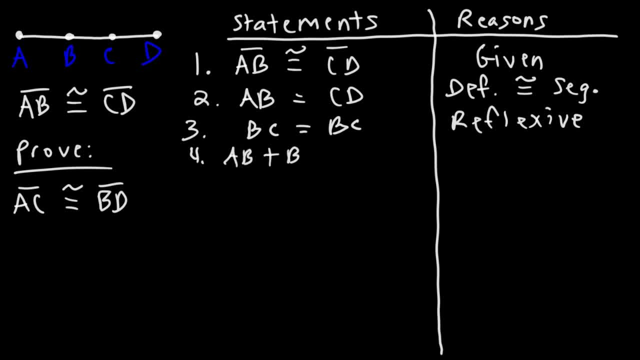 So we're going to get AB plus BC. basically add in the left side and add in the right side. of the two equations We're going to get that's going to equal BC plus CD. Now this is basically the addition. property of equality. 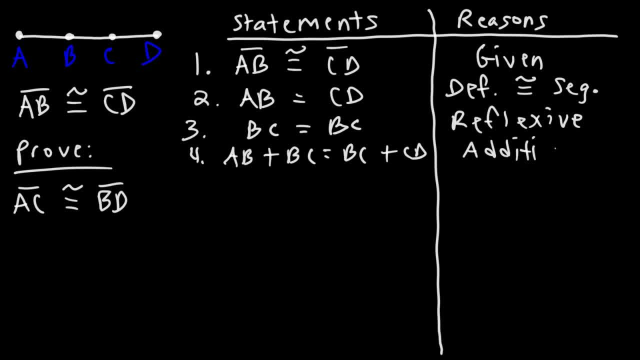 I'm just going to write addition. Now let's move on to step five. So what is AB plus BC equal to? So, as we said before, AB plus BC is AC. So let's make that our statement for number five: AB plus BC is equal to AC. 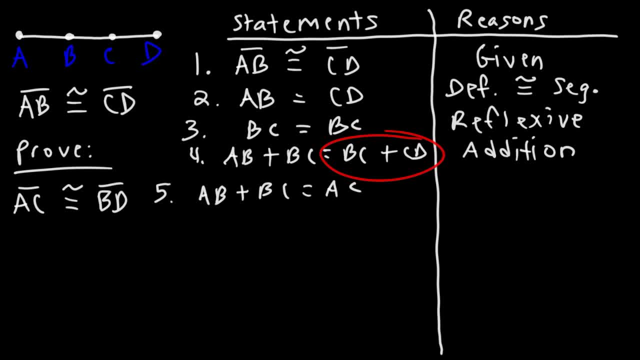 And focusing on the right side of the equation, BC plus CD- that's going to be BD. So let's write that as well. BC plus CD is equal to BD. So what should we write on the right side for this? This is the segment addition postulate. 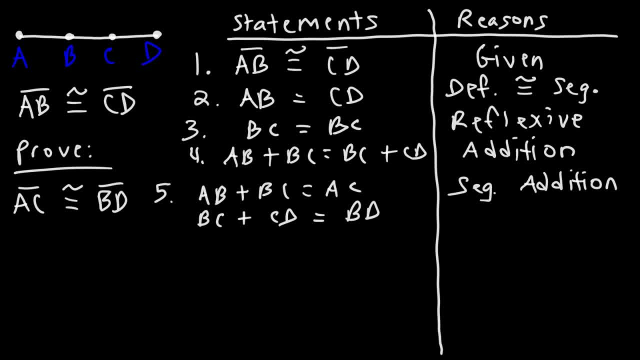 So I'm just going to write segment addition on the right side. So now our next step is to replace. Because AB plus BC is equal to AC in equation four. we're going to replace AB plus BC with AC in step six. 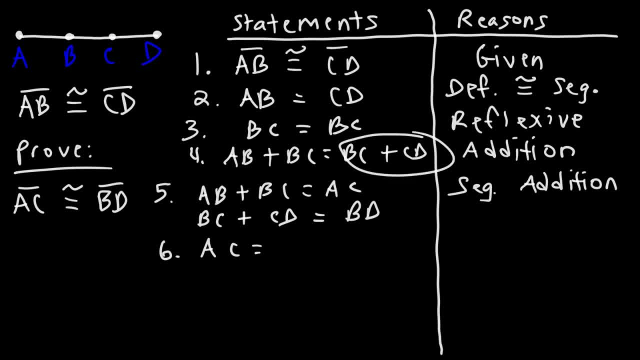 Now BC plus CD is equal to BD, So we're going to substitute BC plus CD with BD, And this is, as you guessed it, the substitution property. Now think about how we went from steps one to two, using definition of congruent segments. 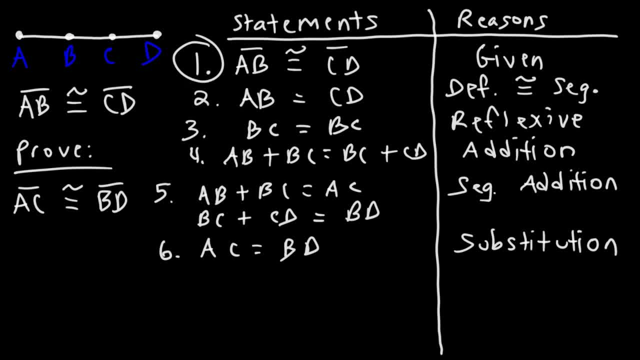 So now we're going to go into reverse order, from statement six to statement seven. If AC is equal to BD, then we could say that segment AC is congruent to segment BD, based on definition of congruent segments. And so that's how we can prove that. 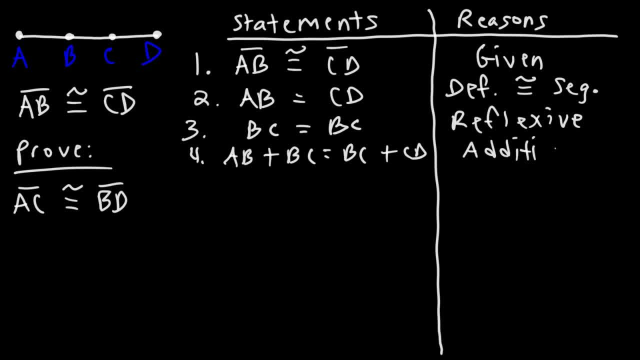 I'm just going to write addition. Now let's move on to step five. So what is AB plus BC equal to? So, as we said before, AB plus BC is AC. So let's make that our statement for number five: AB plus BC is equal to AC. 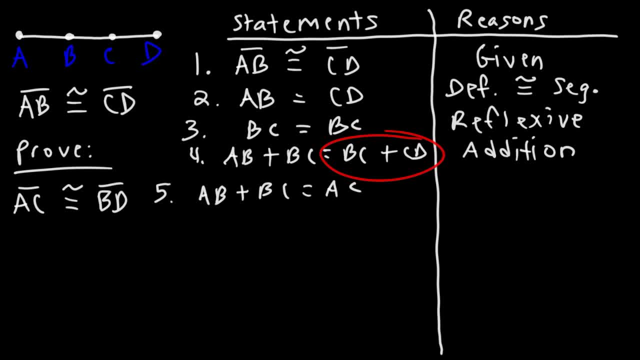 And focusing on the right side of the equation, BC plus CD- that's going to be BD. So let's write that as well. BC plus CD is equal to BD. So what should we write on the right side for this? This is the segment addition postulate. 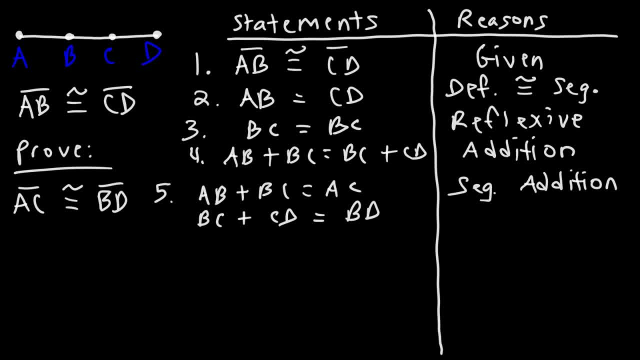 So I'm just going to write segment addition on the right side. So now our next step is to replace. Because AB plus BC is equal to AC in equation four. we're going to replace AB plus BC with AC in step six. 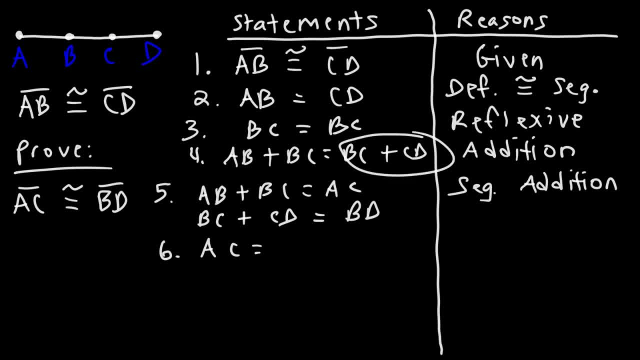 Now BC plus CD is equal to BD, So we're going to substitute BC plus CD with BD, And this is, as you guessed it, the substitution property. Now think about how we went from steps one to two, using definition of congruent segments. 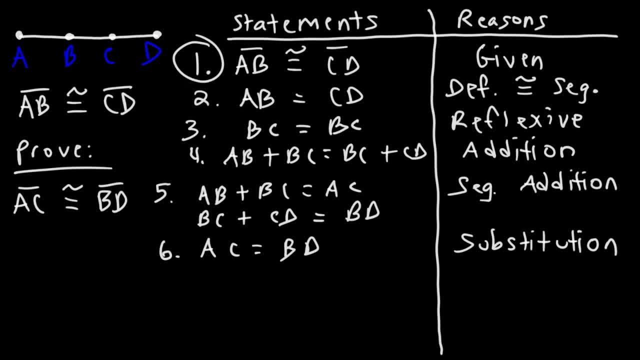 So now we're going to go into reverse order, from statement six to statement seven. If AC is equal to BD, then we could say that segment AC is congruent to segment BD, based on definition of congruent segments, And so that's how we can prove that these two segments are congruent. 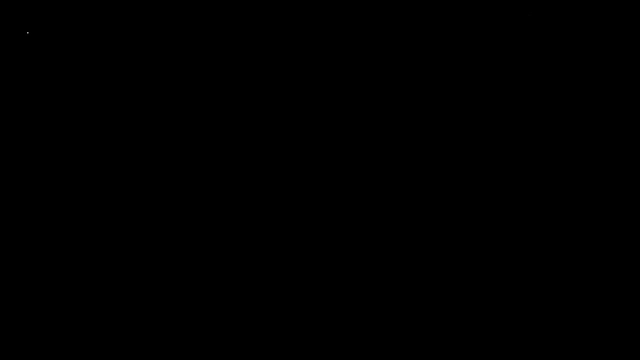 using two column proofs. Now let's work on a similar but different problem And let's change the letters. So we're going to use QRST, Given that segment QS is congruent to segment BD and segment RT, go ahead and prove the following statement: 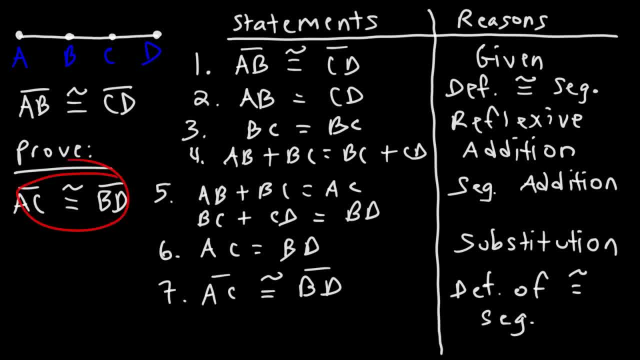 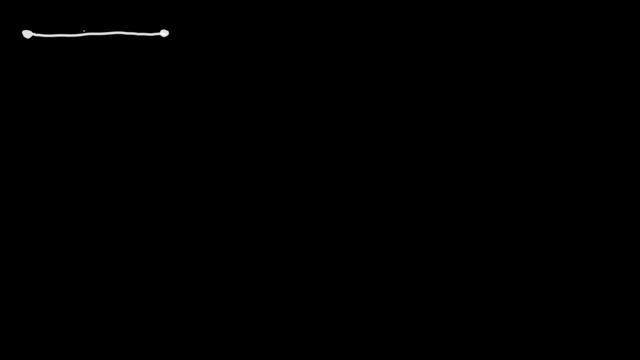 these two segments are congruent using two column proofs. Now let's work on a similar but different problem And let's change the letters. So we're going to use QRST. Given that segment QS is congruent to segment RT, go ahead and prove the following statement: 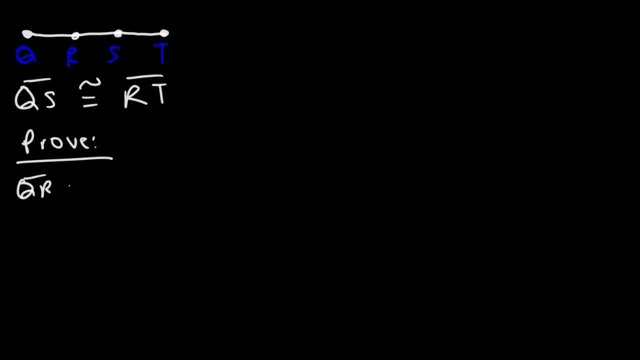 Go ahead and show that segment QR is congruent to segment ST. So this is basically the reverse of the last problem. But feel free to pause the video and work on this example. So number one is going to be what we're given, That is, QS is congruent to RT. 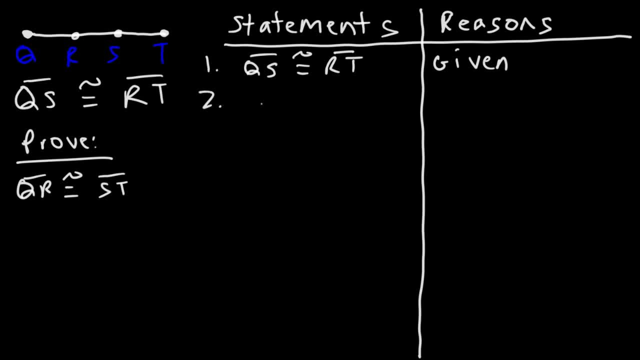 What's our next step? Our next step is saying that QS is equal to RT, And the reason for that is going to be definition of congruent segments. Now let's focus on QS. QS, as we can see, is the sum of QR and RS. 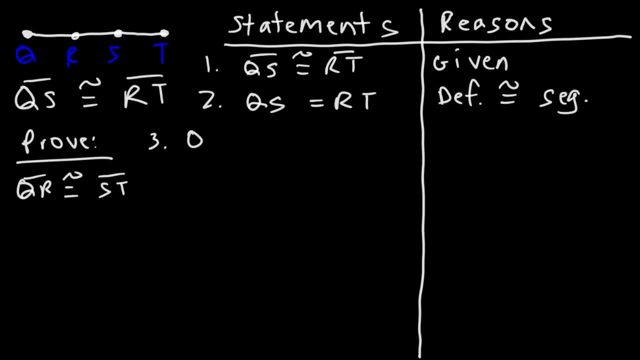 So let's write that in statement three: QS is equal to QR plus RS. Now what about RT? RT is the sum of RS and ST, So RT is equal to RS plus ST. And the reason for this? just like in the last problem. 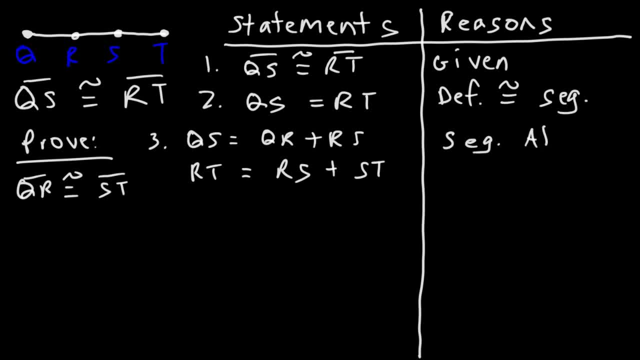 is going to be the segment addition postulate. Now, what's next? The next thing is substitution. We can replace QS with QR plus RS, And then, on the right side of equation two, or the equation that's in statement two, we can replace RT with RS plus ST. 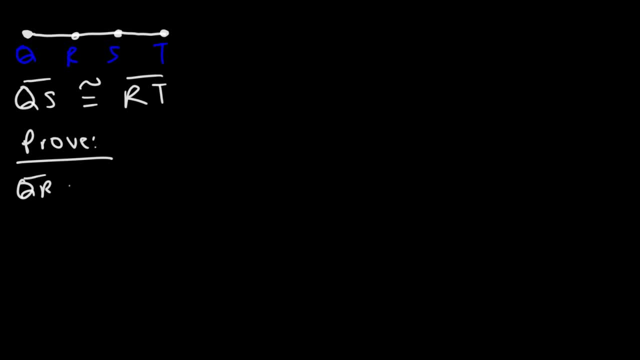 Go ahead and show that segment QR is congruent to segment ST. So this is basically the reverse of the last problem. But feel free to pause the video and work on this example. So number one is going to be what we're given, That is, QS is congruent to RT. 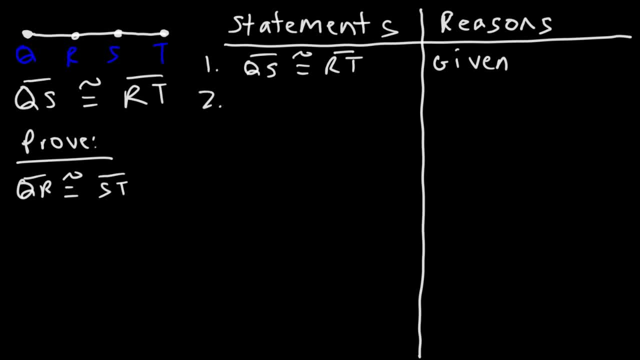 What's our next step? Our next step is saying that QS is equal to RT, And the reason for that is, and the reason for that is going to be, definition of congruent segments. Now let's focus on QS. QS, as we can see, is the sum of QR and RS. 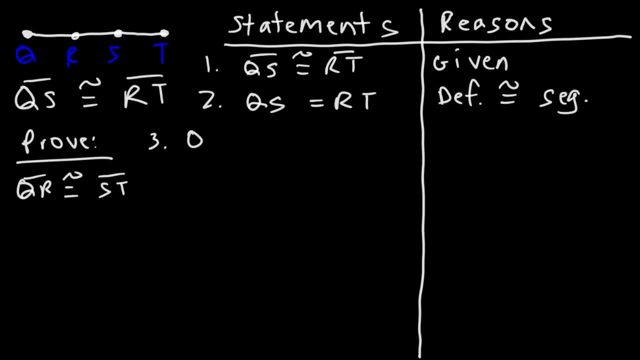 So let's write that in statement three: QS is equal to QR plus RS. Now what about RT? RT is the sum of RS and ST, So RT is equal to RS plus ST. And the reason for this? just like in the last problem. 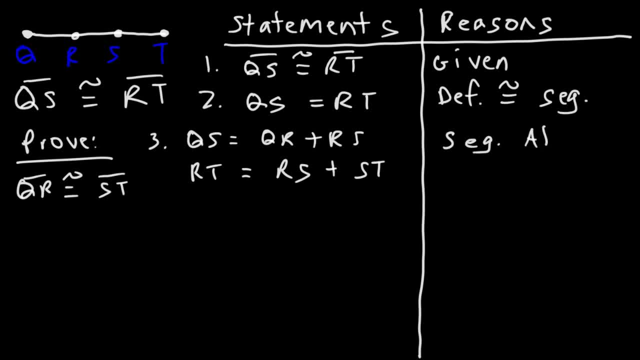 is going to be the segment addition postulate. Now, what's next? The next thing is substitution. We can replace QS with QR plus RS, And then, on the right side of equation two, or the equation that's in statement two, we can replace RT with RS plus ST. 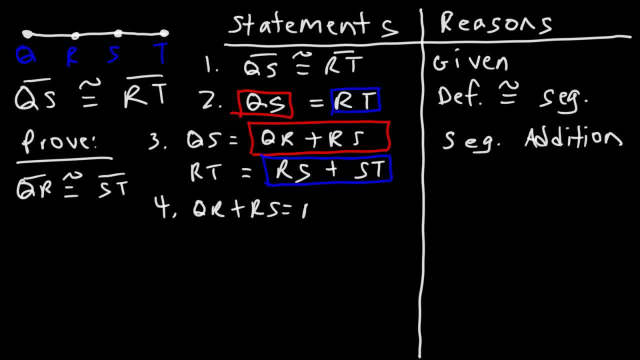 So this is going to be substitution. Now notice that we have RS on both sides. So in order to get QR equal to ST, which we have here, we need to subtract both sides. So in order to get QR equal to ST, which we have here, 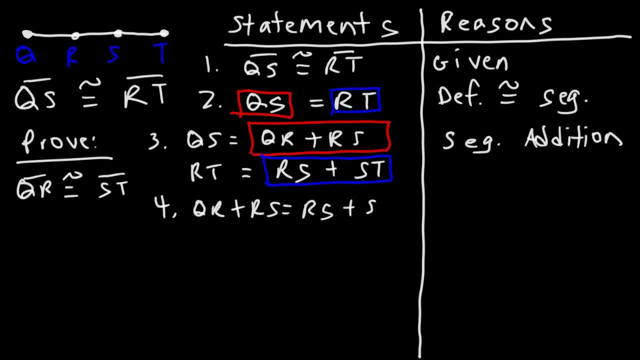 RT is equal to RS plus ST, So this is going to be substitution. Now notice that we have RS on both sides. So in order to get QR equal to ST, which we have here, we need to subtract both sides by RS. 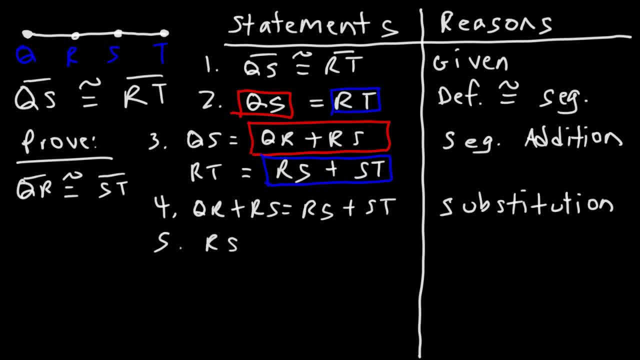 Before we do that, let's write down another formality. Let's say: RS is equal to itself, based on the reflexive property. Now we're going to take statement four and subtract it by statement five, So these two will cancel and we're going to have: QR is equal to ST. 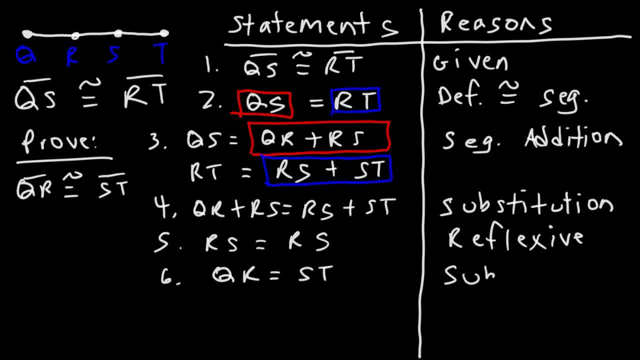 And this is based on the subtraction property. Now our final step, step seven, is to say that segment QR is congruent to segment ST, based on definition of congruent segments, And so that's how we can show that these two segments are congruent to each other. 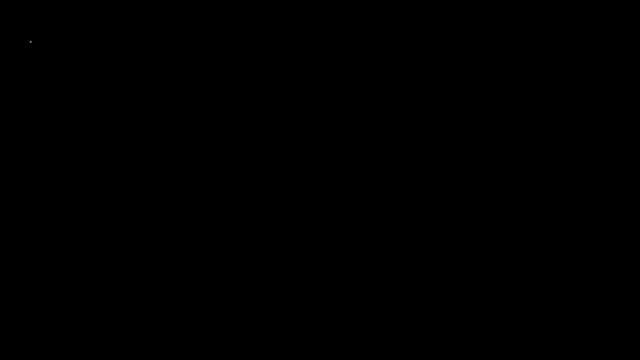 using two column proofs. Now let's work on another example. So let's say we have two separate segments. The first one will have the letters A, B and C and the second one D, E, F. So let's say that we're given. 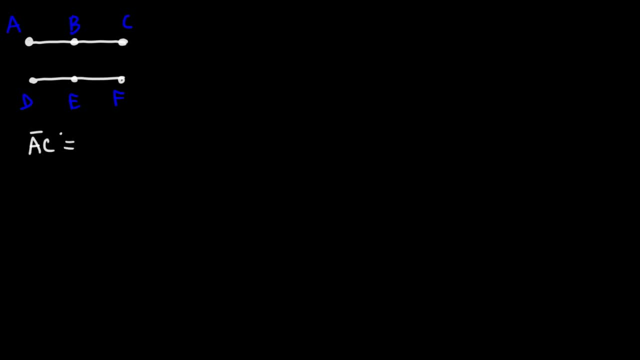 that AC is congruent to DF, and let's say that B is the midpoint of segment AC and we're also given that E is the midpoint of segment DF. Your task is to prove that segment AB is congruent to segment DE. So let's think about what we have. 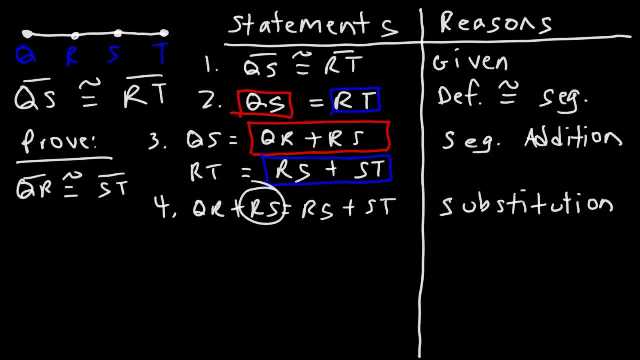 we need to subtract both sides by RS. Before we do that, let's write down another formality. Let's say RS is equal to itself, based on the reflexive property. Now we're going to take statement four and subtract it by statement five. 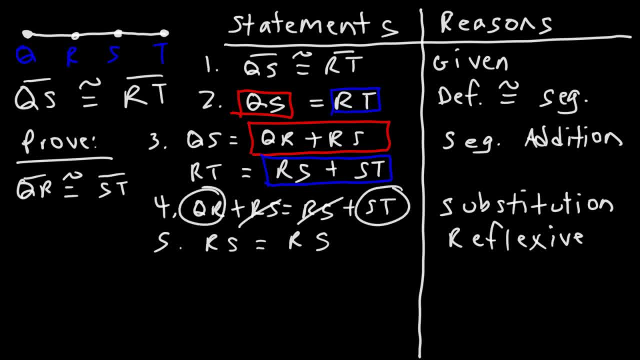 So these two will cancel and we're going to have: QR is equal to ST And this is based on the subtraction property. Now our final step, step seven, is to say that segment QR is congruent to segment ST, based on definition of congruent segments. 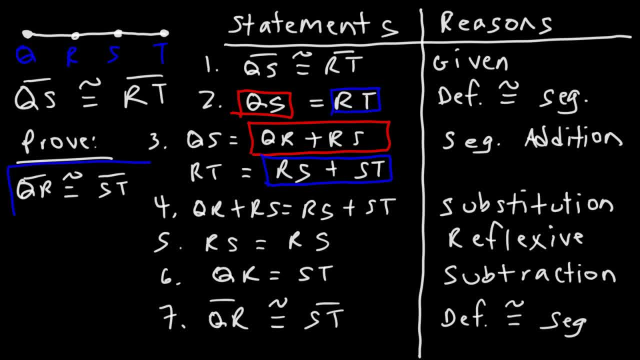 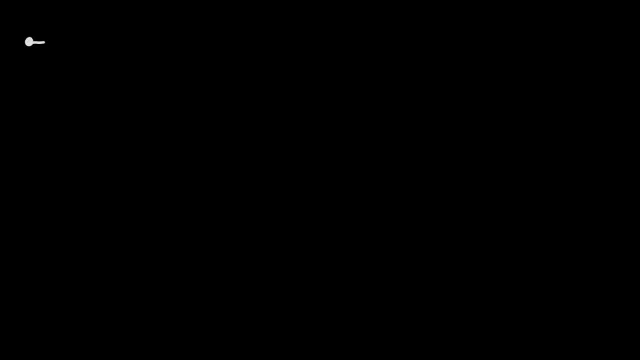 And so that's how we can show that these two segments are congruent to each other, Using two column proofs. Now let's work on another example. So let's say we have two separate segments. The first one will have the letters A, B and C. 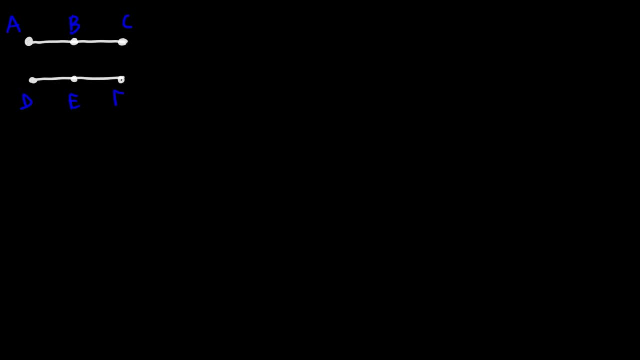 and the second one, D, E, F. So let's say that we're given that AC is congruent to D- F And let's say that B is the midpoint of segment AC And we're also given that E is the midpoint. 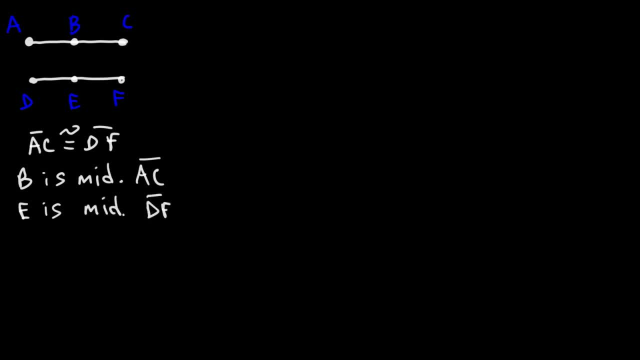 of segment D F. Your task is to prove that segment AB is congruent to segment D E. So let's think about what we have. We're told that AC is congruent to D F And our goal is to show that AB. 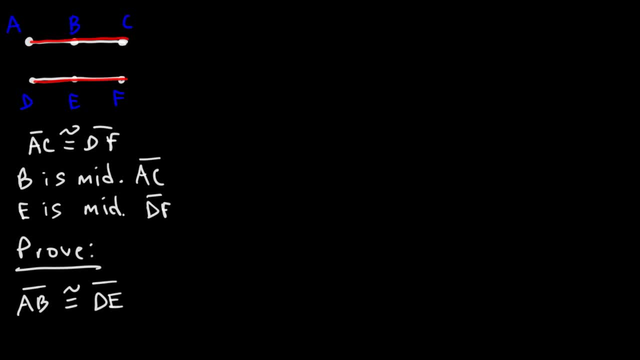 We're told that AC is congruent to DF and our goal is to show that AB is congruent to DE. So go ahead and work on this example. Write up a two column proof to show that AB is congruent to DE. Write up a two column proof. 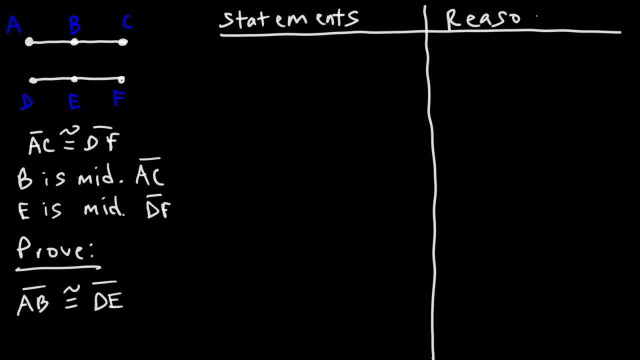 to show that AB is congruent to DE. Write up a two column proof to show that AB is congruent to DE. So let's start with the first one. So let's start with the first one. AC is congruent to DF. 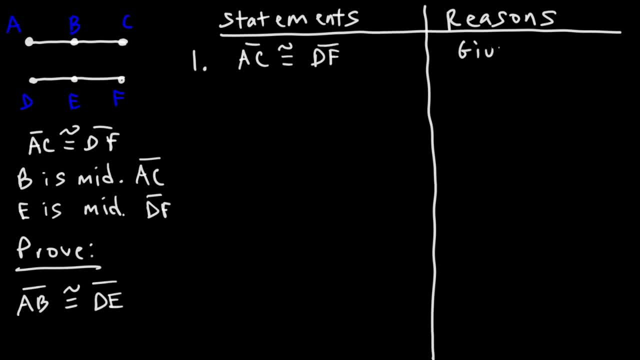 AC is congruent to DF. That's given. Our second given statement is that B is the midpoint of segment AC. is that B is the midpoint of segment AC? and then our third given statement is that E is the midpoint of segment DF. now, 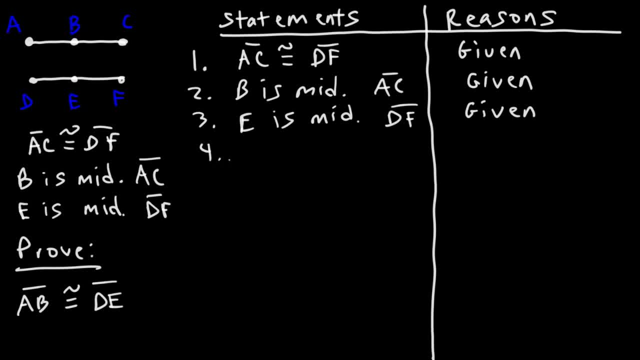 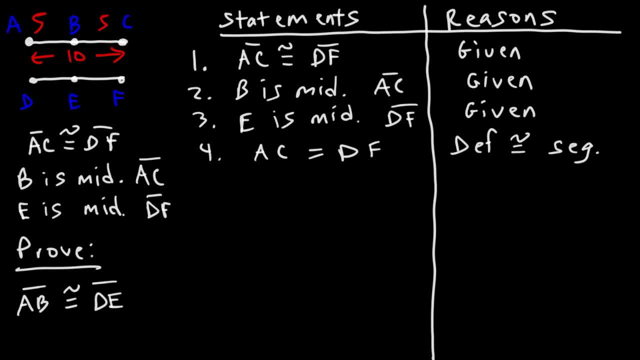 and B is the midpoint, that means a, B and and B is the midpoint, that means a, B and BC has to be 5, just for the sake of BC has to be 5, just for the sake of BC has to be 5, just for the sake of example. 5 is 1. half of 10. 5 corresponds. 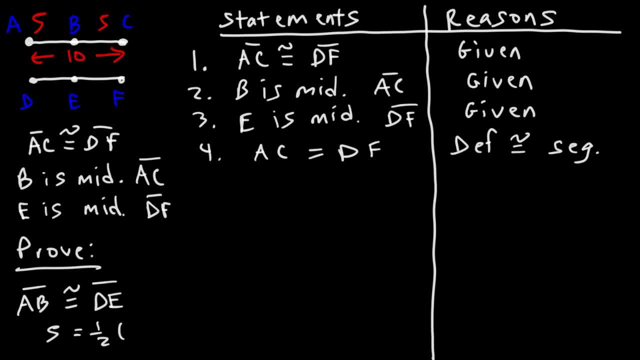 example 5 is 1 half of 10. 5 corresponds. example 5 is 1 half of 10. 5 corresponds to a B. 10 corresponds to AC. so we could to a B 10 corresponds to AC. so we could to a B: 10 corresponds to AC. so we could say that. just to think about the whole. 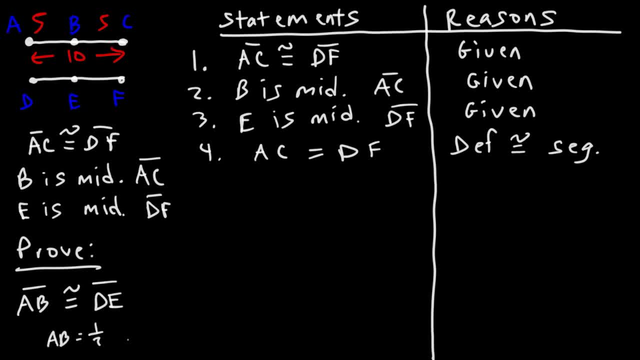 say that just to think about the whole. say that, just to think about the whole situation. we can say that a- B is one situation. we can say that a- B is one situation. we can say that a- B is one half of AC. but before we do that, let's 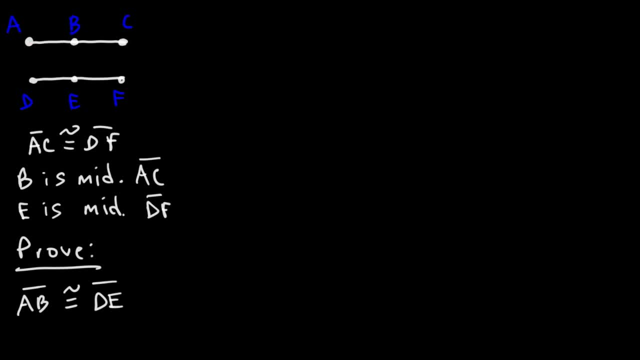 is congruent to D E. So go ahead and work on this example. Write up a two column proof to show that AB is congruent to D E. So let's start with the first one: AC is congruent to D F. 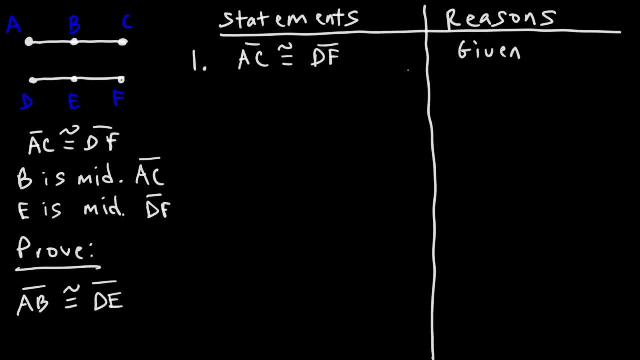 That's given. Our second given statement is that B is the midpoint of segment AC, And then our third given statement is that E is the midpoint of segment D F. Now, what else can we say? Well, if segment AC is congruent to segment D F, 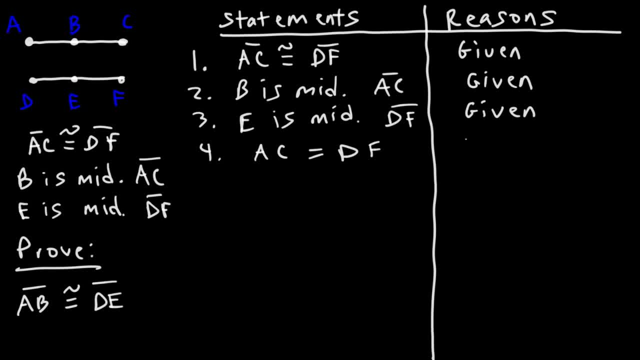 we could say that AC is equal to D, F, based on definition of congruent segments. Now remember, we're trying to make these two equal to each other And it stands to reason that AB is going to be one half of AC. Let's say, if AC 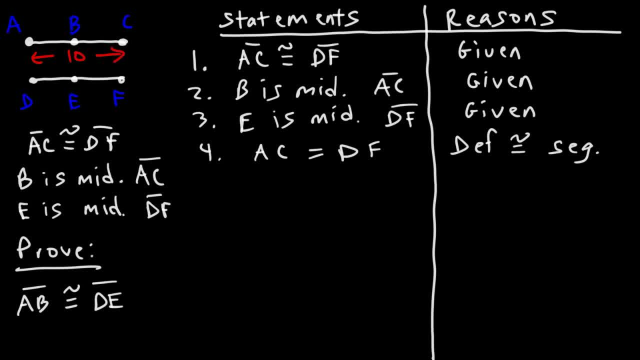 is 10 units long And B is the midpoint. That means AB and BC has to be five. Just for the sake of example, Five is one half of 10.. Five corresponds to AB, 10 corresponds to AC. So we could say that. 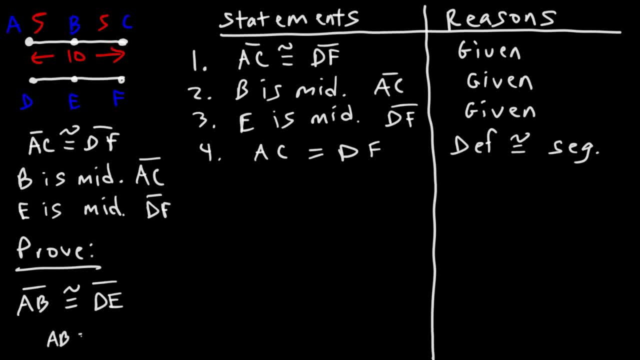 just to think about the whole situation, we could say that AB is one half of AC. But before we do that, let's focus on statement two and divide this equation by two. If we divide both sides by two, we'll get this equation. 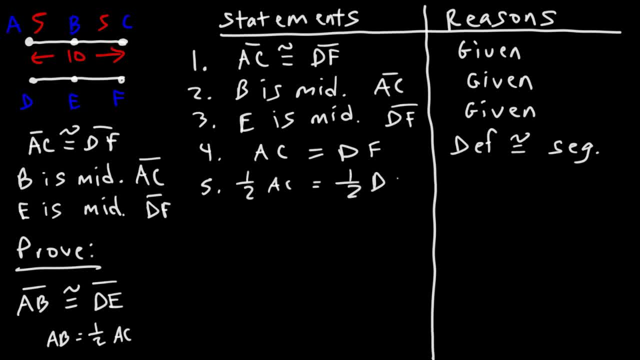 One half AC is equal to one half D F. Now what's the reason for this? Since we divided both sides by a number, we could say that this is due to the division property. Now what's our next step? Notice that we could replace. 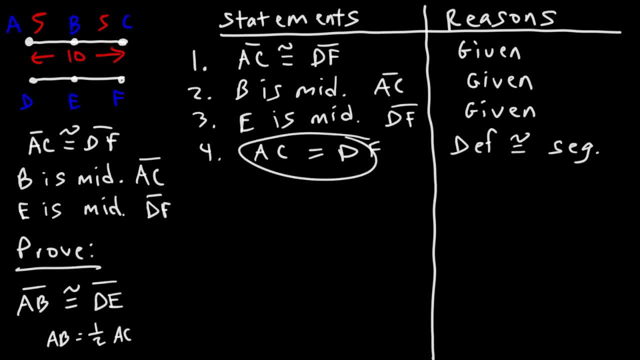 half of AC. but before we do that, let's half of AC. but before we do that, let's focus on statement 2 and divide this focus on statement 2 and divide this focus on statement 2 and divide this equation by 2 if we divide both sides by. 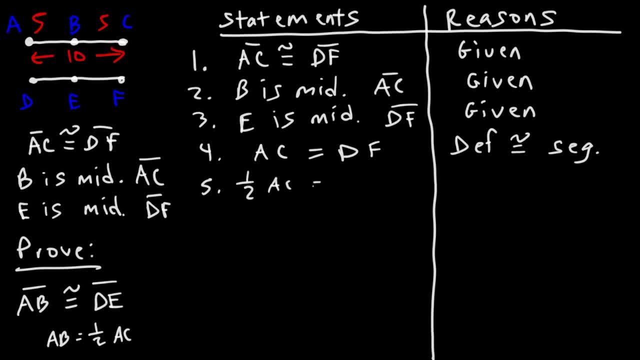 equation by 2. if we divide both sides by equation by 2, if we divide both sides by 2, we'll get this equation: 1 half AC is 2, we'll get this equation: 1 half AC is 2. we'll get this equation: 1 half AC is equal to 1 half DF. now what's the reason? 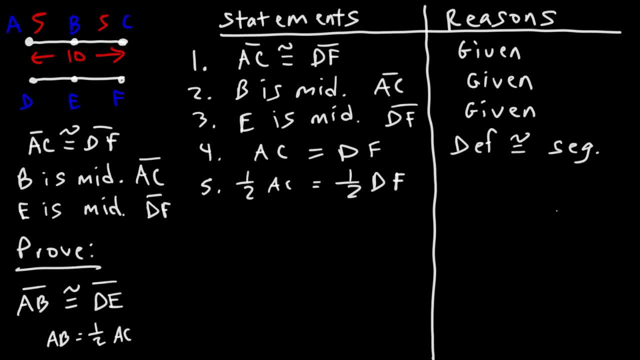 equal to 1 half DF. now what's the reason? equal to 1 half DF, now. what's the reason for this? since we divided both sides by for this, since we divided both sides by for this, since we divided both sides by a number, we could say that this is due. 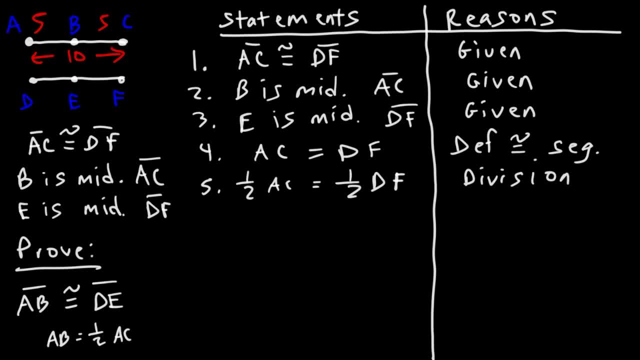 a number. we could say that this is due a number. we could say that this is due to the division property. now, what's our to the division property now? what's our to the division property now? what's our next step? notice that we can replace 1. 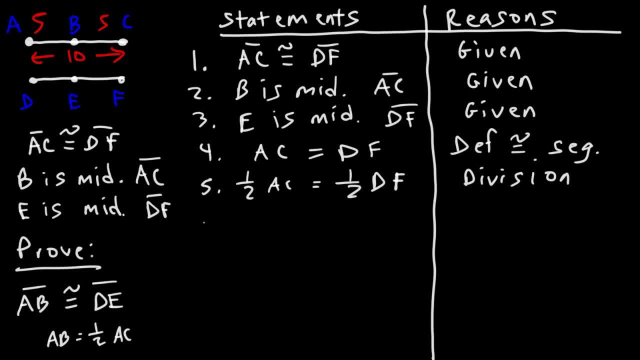 next step: notice that we can replace 1. next step: notice that we can replace 1 half AC with a B. but before we do that, half AC with a B, but before we do that, half AC with a B- but before we do that we need to say that a- B is equal to 1. 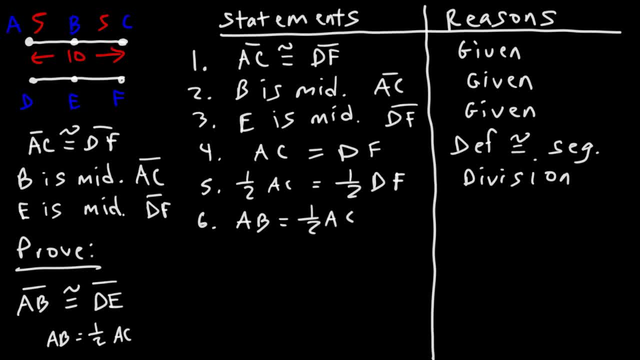 we need to say that a B is equal to 1. we need to say that a B is equal to 1 half AC, and likewise we can also say half AC, and likewise we can also say half AC, and likewise we can also say that de is 1 half of DF. now, why can we? 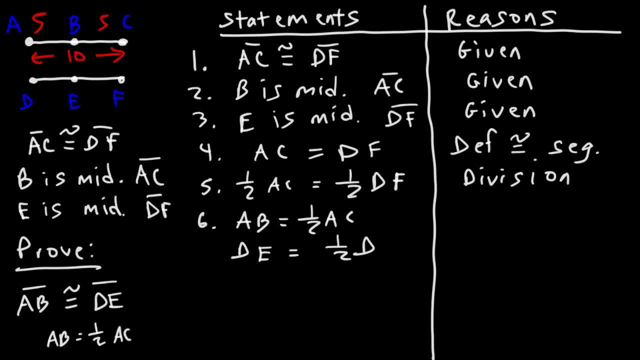 that de is 1 half of DF now. why can we that de is 1 half of DF now? why can we say these things? how do we get this, say these things? how do we get this, say these things? how do we get this information, information, information. 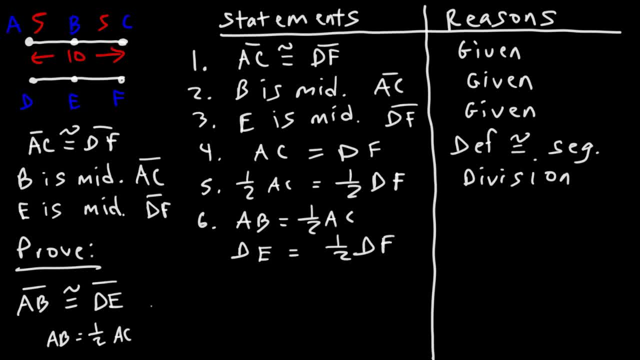 information, information. well, we realized that a B was 1 half of. well, we realized that a B was 1 half of. well, we realized that a B was 1 half of AC because B was the midpoint of AC. so AC because B was the midpoint of AC. so 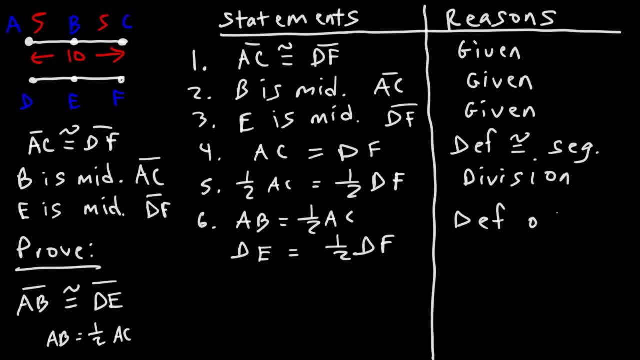 AC because B was the midpoint of AC. so therefore, this is due to definition of. therefore, this is due to definition of. therefore, this is due to definition of midpoint. now we can substitute 1 half AC midpoint. now we can substitute 1 half AC midpoint. now we can substitute 1 half AC with a- B. so in step 5 we're replacing. 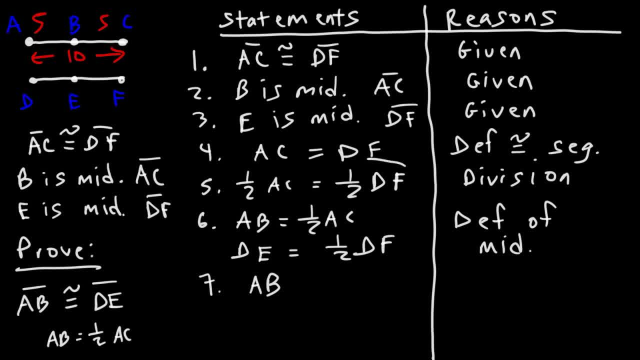 with a B. so in step 5 we're replacing with a B. so in step 5 we're replacing or substituting, or substituting, or substituting 1 half AC with a B and we're going to replace 1 half of DF, 1 half AC with a B, and we're going to replace 1 half of DF. 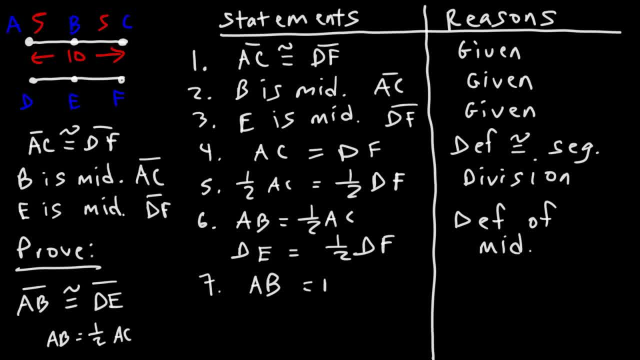 1 half AC with a B and we're going to replace 1 half of DF with de. so we have a B is equal to with de. so we have a B is equal to with de. so we have a B is equal to de, and this is due to the substitution. 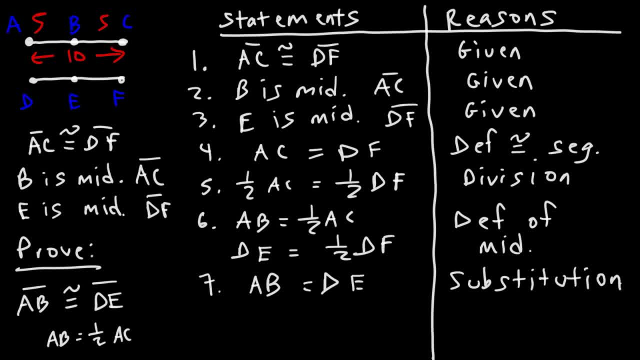 de and this is due to the substitution de and this is due to the substitution property. now step 8, our last step. we property. now step 8, our last step. we property, now step 8, our last step. we could say that a, B is congruent to de. 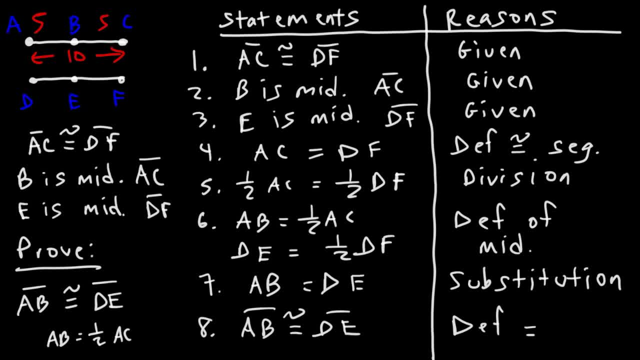 could say that a- B is congruent to de, could say that a- B is congruent to de based on definition of congruent, based on definition of congruent, based on definition of congruent segments, and that's basically it so: segments, and that's basically it so. 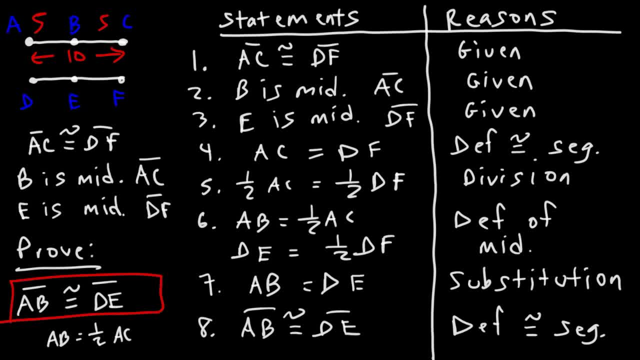 segments and that's basically it. so that's how you can prove that these two, that's how you can prove that these two, that's how you can prove that these two segments are congruent to each other. so segments are congruent to each other, so segments are congruent to each other. so that's it for this video, if you like it. 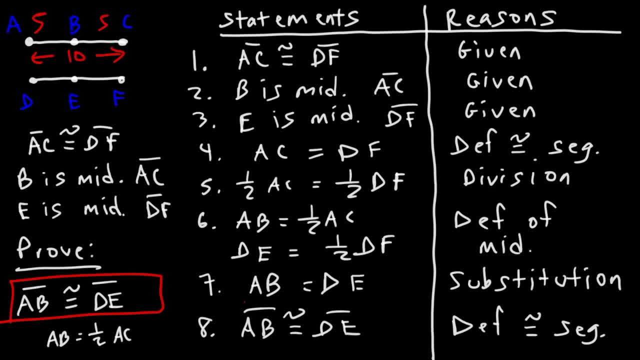 that's it for this video, if you like it. that's it for this video. if you like it, don't forget to subscribe. and thanks, don't forget to subscribe. and thanks, don't forget to subscribe. and thanks again for watching. 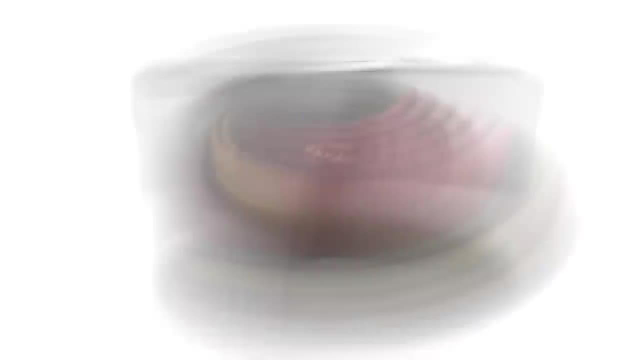 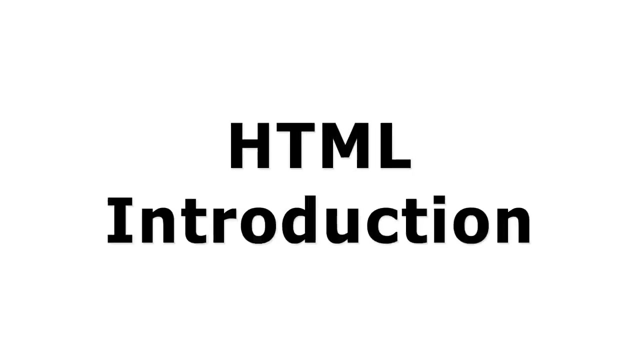 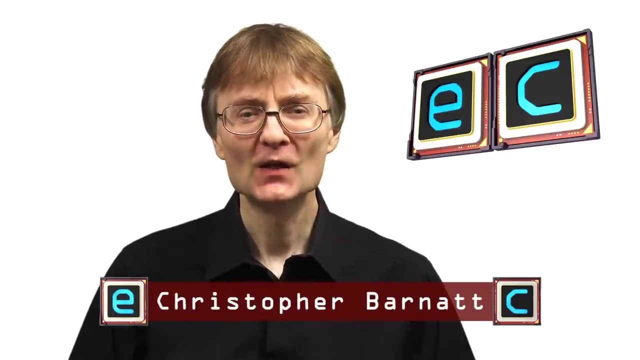 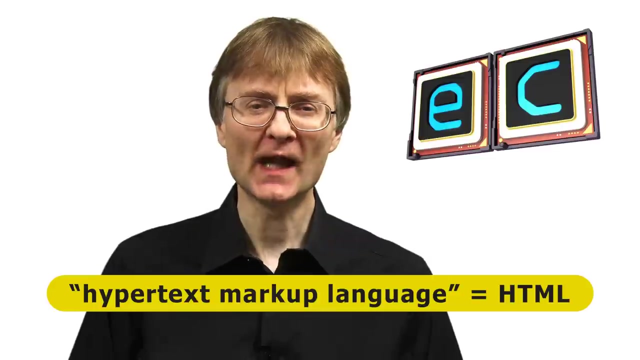 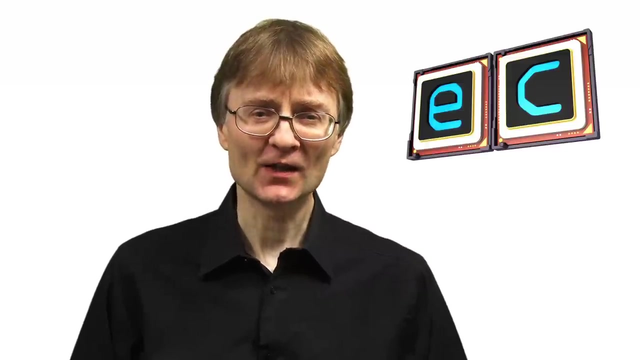 Welcome to another video from ExplainingComputerscom. This time, I'm going to show you how to write a simple web page using the Hypertext Markup Language or HTML. All you need to follow this through is a web browser and access to a text editor such as Notepad, which is included. 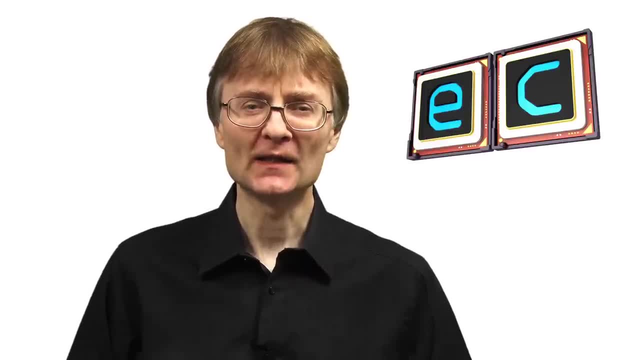 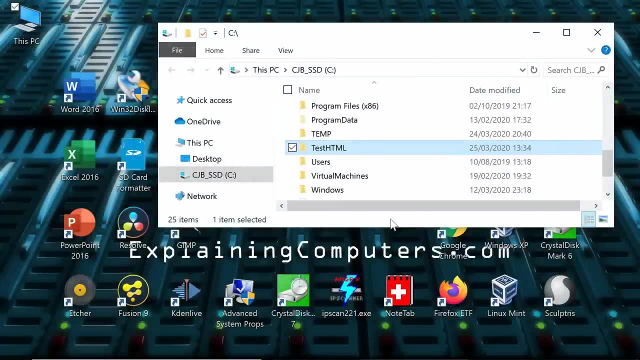 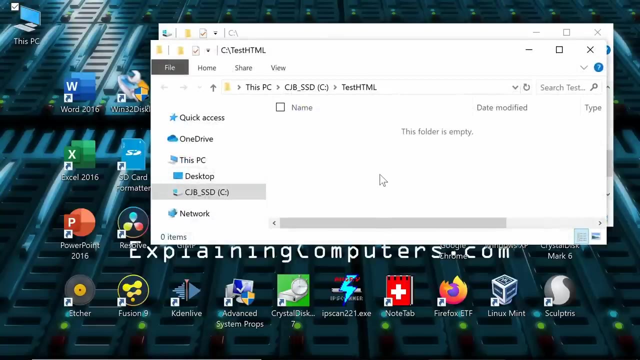 with Windows. So let's go and get started. So here we are in Windows, where on my C drive, I've created a directory called TestHTML where we're going to store the content we create in this video. So I'm going to go down. 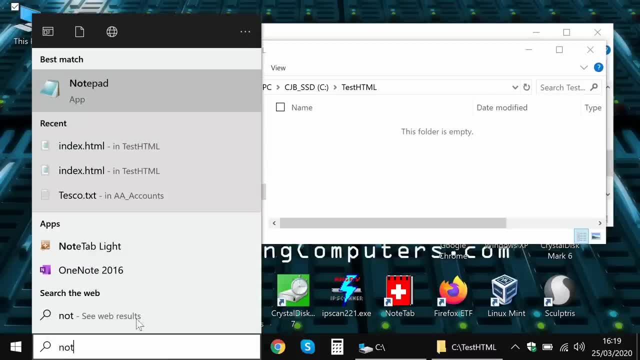 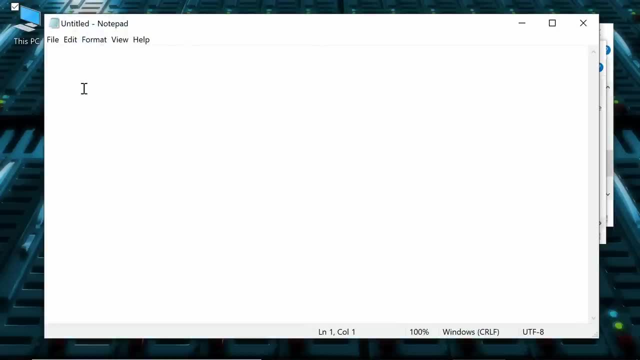 and launch Notepad. We'll just type a Notepad in there and it'll come up. There it is As I said in the introduction. you can do everything here with Notepad. You could use more complicated editors, but Notepad will be fine for our purposes And here under Format.